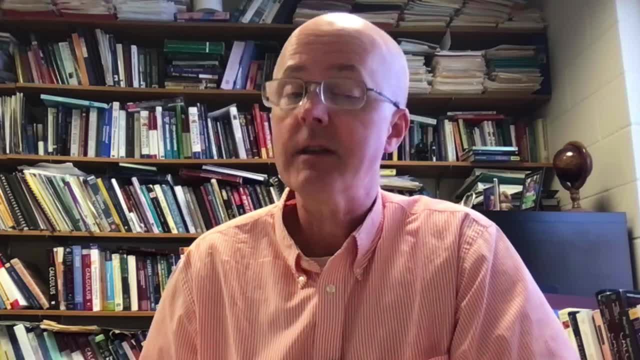 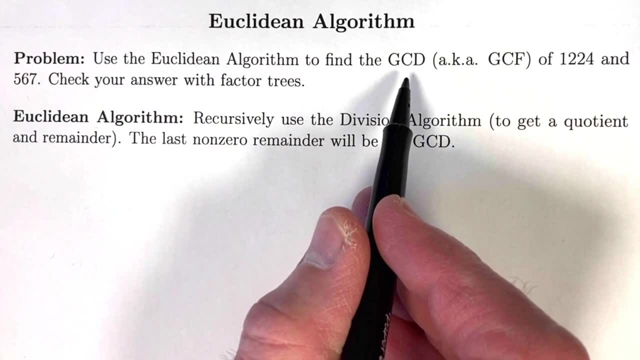 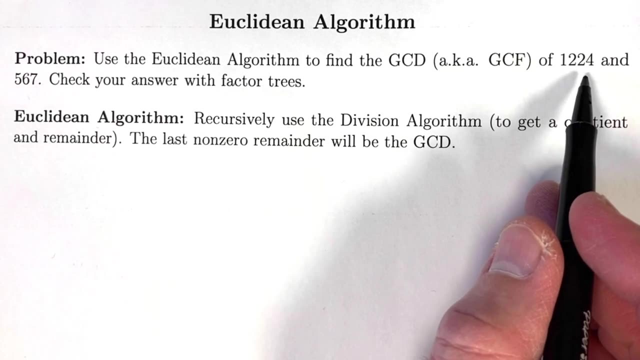 The Euclidean algorithm is an ancient method to find the greatest common divisor of two whole numbers. This problem says to use the Euclidean algorithm to find the GCD greatest common divisor, also known as GCF for greatest common factor, of the two whole numbers 1224 and 567. and then we'll 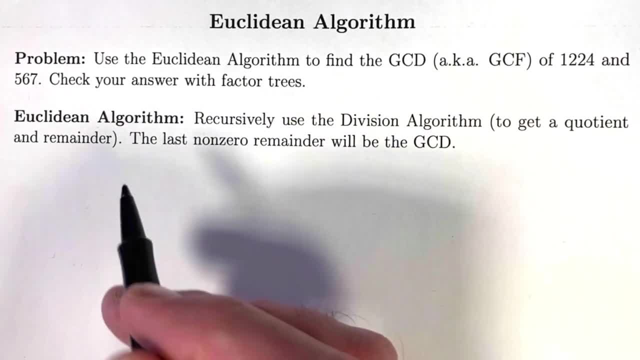 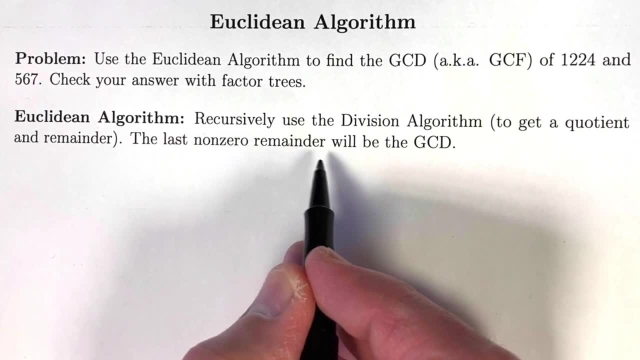 check our answer with factor trees. What is the Euclidean algorithm? We recursively use the division algorithm, where we get a quotient and remainder, and the last non-zero remainder will be the GCD, the greatest common divisor. So start by taking the bigger number, 1224. 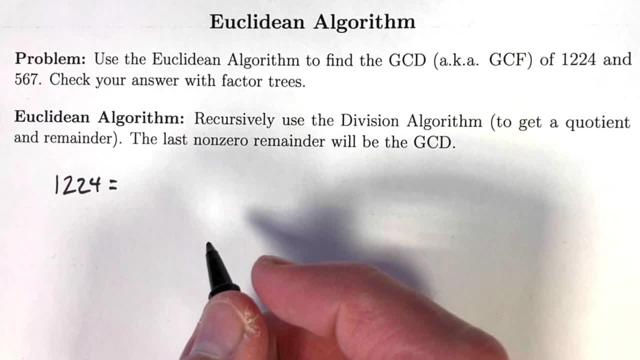 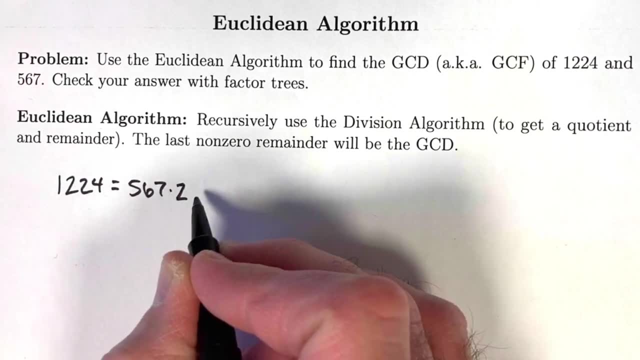 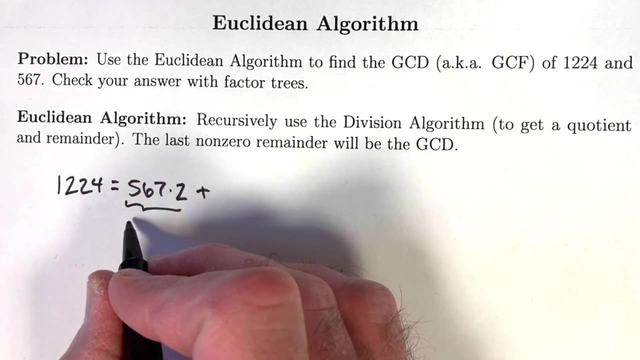 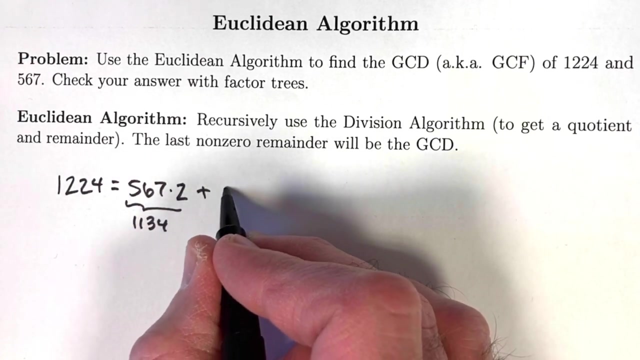 and dividing it by the smaller number, 567.. 567 goes into 1224. twice the quotient is two. What is the remainder that we need to add to this to get 1224?? 567 times two is 1134.. We need to add 90 to that to get 1224.. 90 is the remainder. 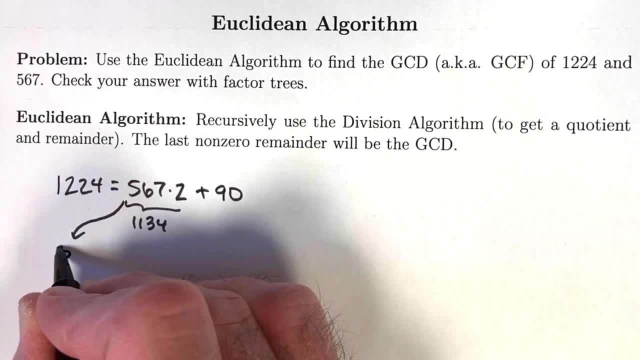 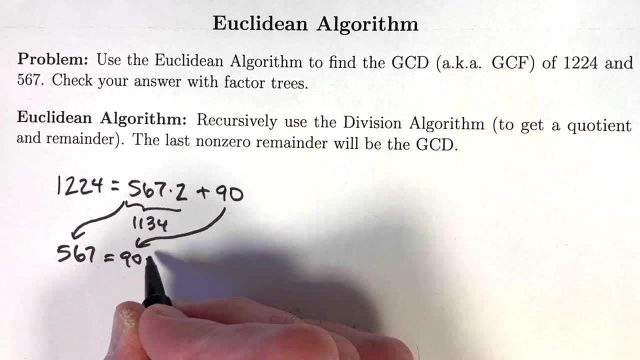 Now take the 567, put it over here and divide it by the remainder 90.. 90 goes into 567. six times 90 times 6 is 540 and the remainder is 27.. Continue that process: take the 90 and divide it by the remainder. 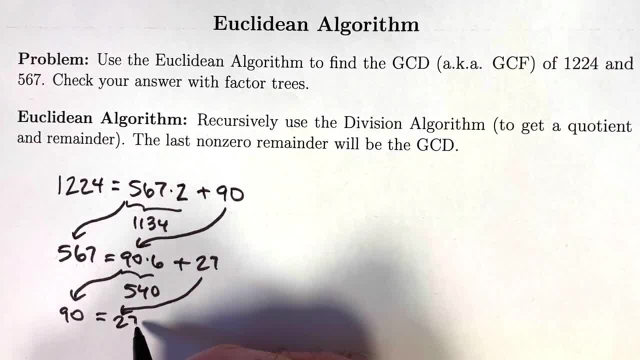 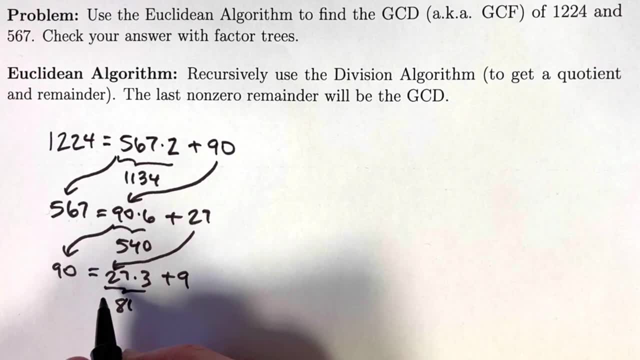 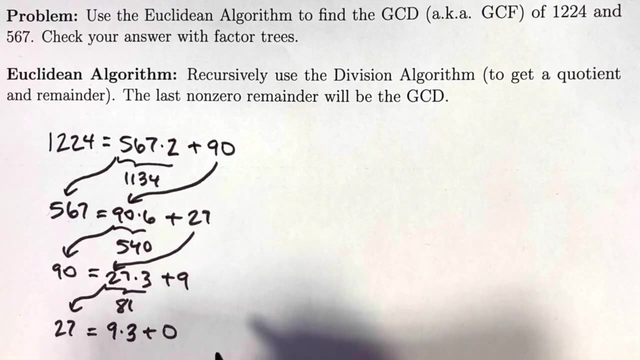 by 27.. 27 goes into 93 times 27 times 3 is 81 with a remainder of 9.. One more step, and we'll be done: 27,, when we divide it by 9, is 9 times 3 with a remainder of 0.. As said, 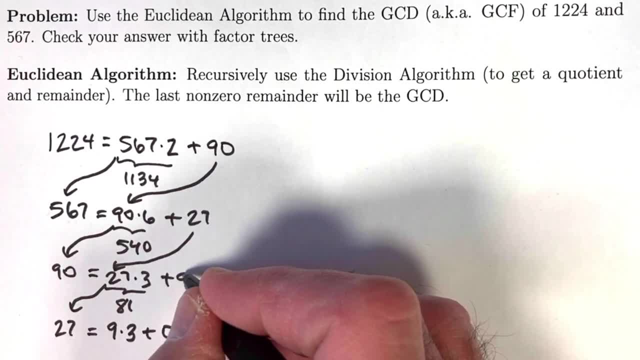 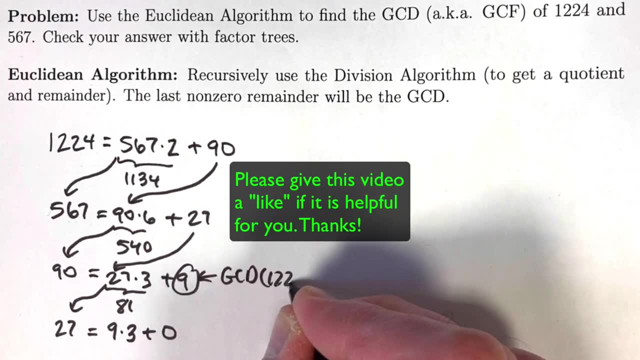 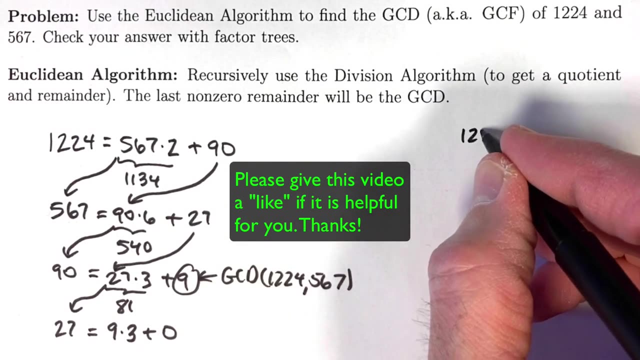 here. the last non-zero remainder will be the GCD. 9 is the last non-zero remainder. This is the answer. This is the GCD of 1,224 and 567.. Now let's check the answer with factor trees. Take 1,224.. First notice: it's an even number. It's divisible by 2.. It's 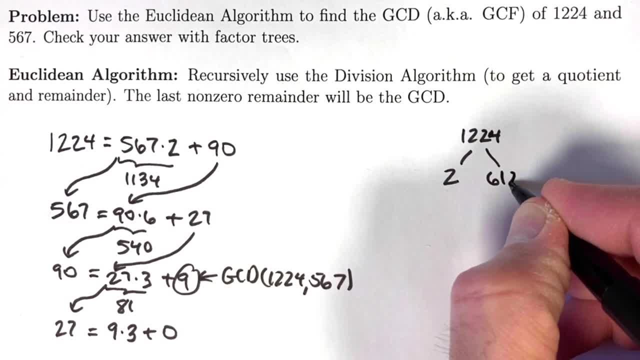 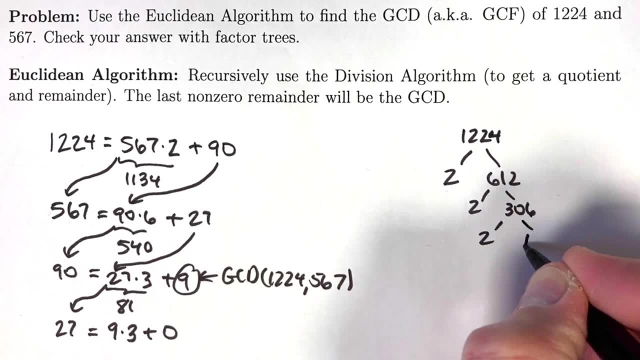 2 times 612.. That is also an even number. It's 2 times 306.. That's also even. It's 2 times 153.. Now, that's an odd number, but it is divisible by 3.. 1 plus 5 plus. 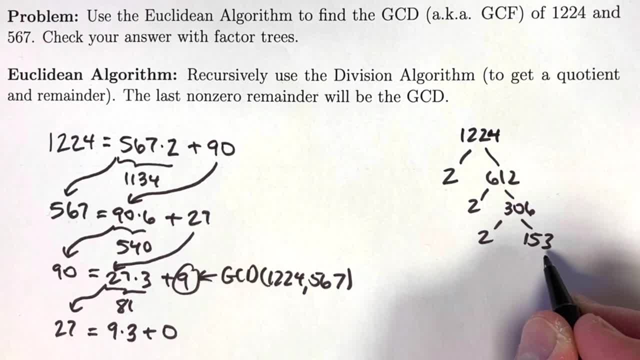 3 is 9.. The sum of the digits is 9.. It's divisible by 3 because 9 is divisible by 3.. It's also divisible by 9,, in fact, because 9 is divisible by 9.. This is going to be 3 times 51, and 51 is 3. 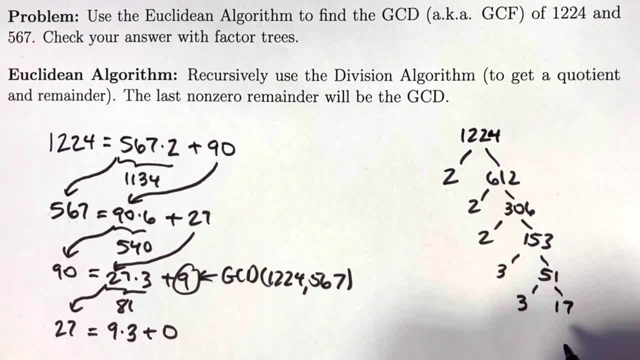 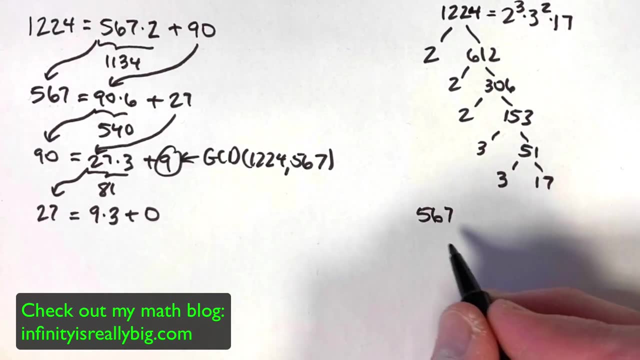 times 17.. The prime factorization of 1,224 is 2 to the third power times 3 to the second power times 17.. Now do the same kind of thing with the other number, 567.. 567 is not even. It's not. 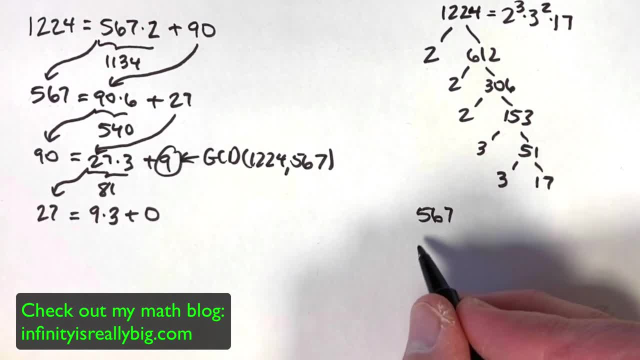 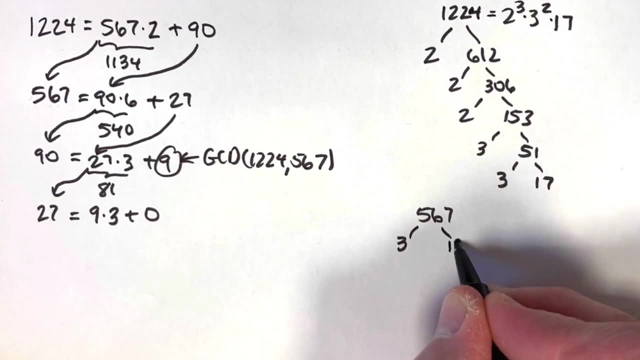 divisible by 2,, but if you add its digits, you get 18,, which is divisible by both 3 and 9.. This is going to be divisible by 9.. It's 3 times 189.. 189 is 3 times 63.. 63 is still divisible by 3.. It's 3. 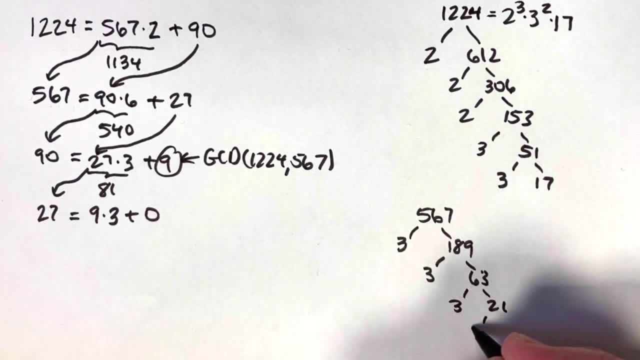 times 21.. 21 is divisible by 3. It's 3 times 7.. Those are all prime numbers. The prime factorization of 567 is 3 to the fourth power times 7.. What primes do these factorizations have in common? They have two factors of 3 in common: 3 squared. 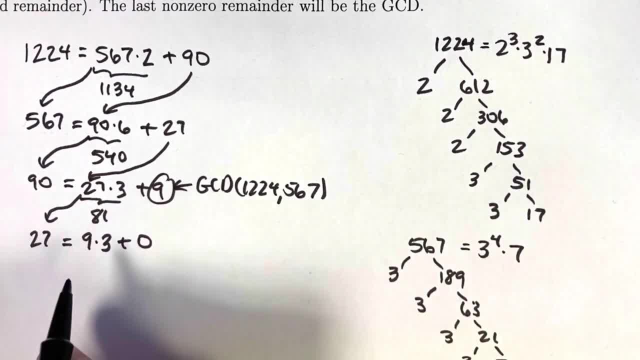 is 9.. 9 is the GCD. You might wonder: why did the Euclidean algorithm work? Why is 9 the GCD based on this method? First of all, 9 certainly is a divisor or a factor of both 1,224 and 567.. 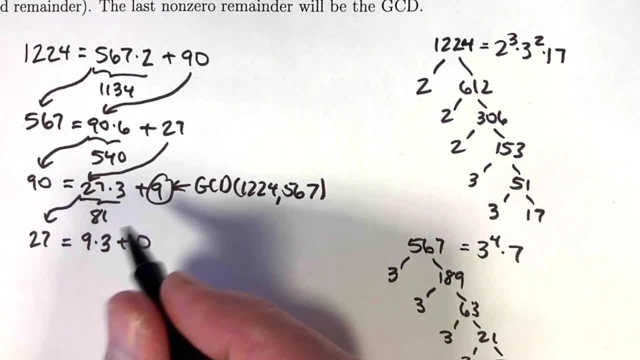 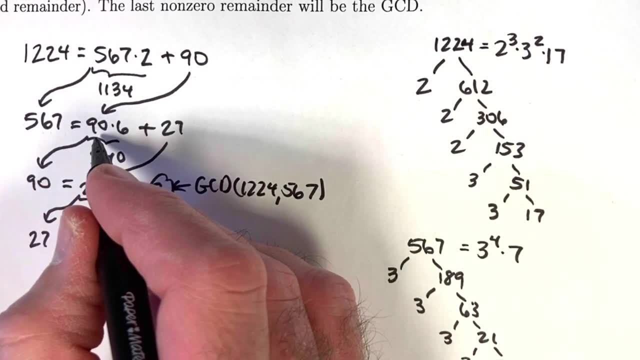 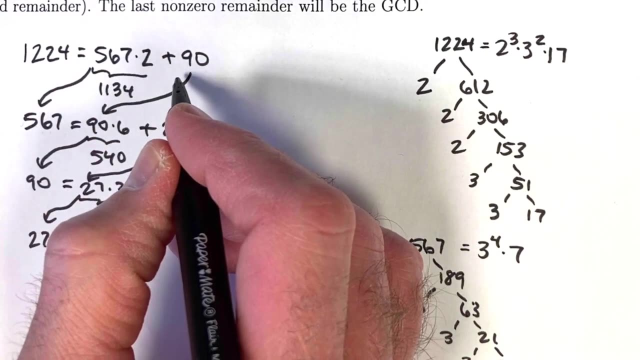 27 is 9 times 7. So 9 divides 27.. 9 also divides 90, because 9 divides both 9 and 27.. 9 also divides 567, because it divides 90 and 27.. And finally, 9 divides 1,224, because it divides 567 and 90.. That's why. 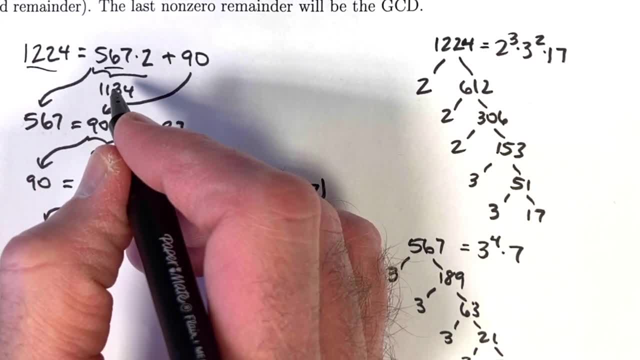 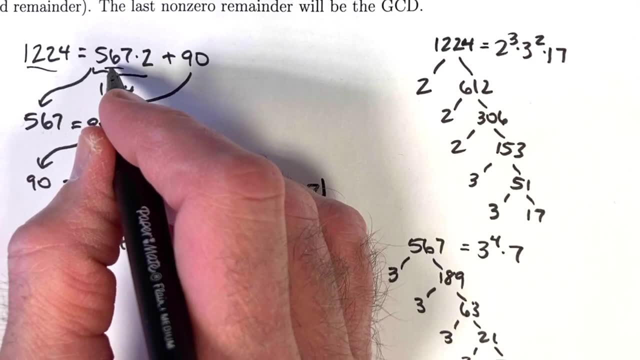 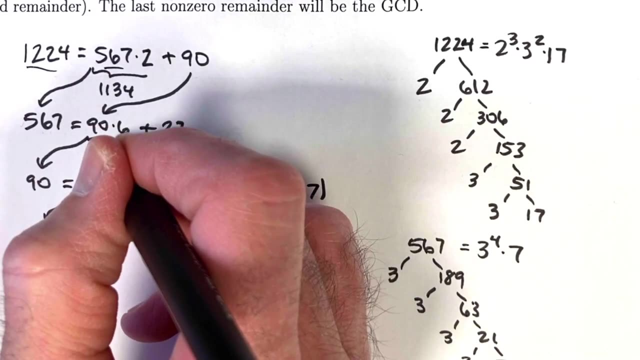 9 is a divisor of both of these numbers. Why is that the greatest common divisor? Because of this first equation. any given divisor of 1,224 and 567 will also divide 90 by solving this equation. So it will also divide 27 by solving this equation for 27.. So it will also divide 9 by solving this. 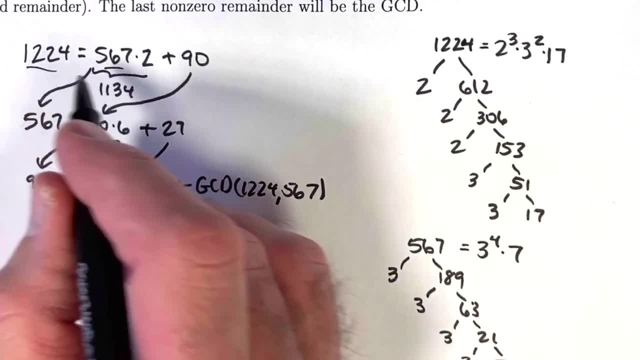 equation for 9.. Any common divisor of 1,224 and 567 must divide 9.. Therefore, 9 must be the greatest common divisor. Thanks for watching.